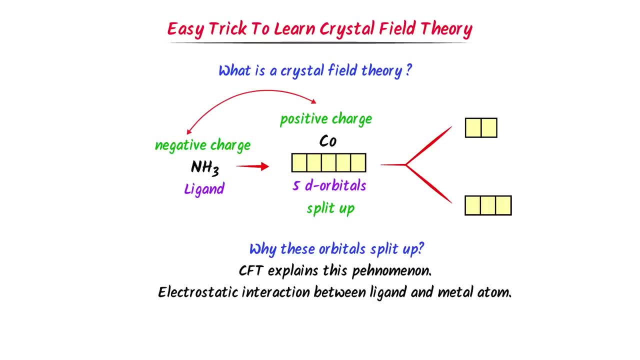 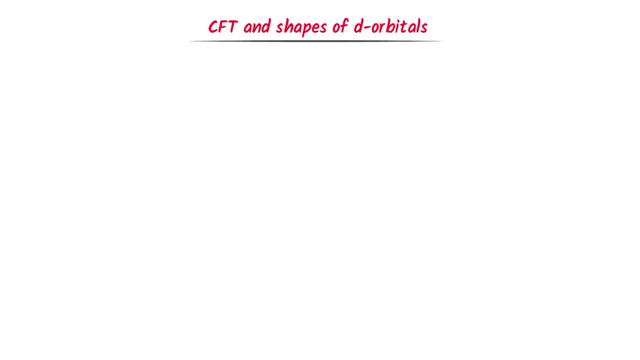 Now to learn captured field theory completely. firstly, we have to learn the shape of the orbitals. We know that d orbitals have 5d. generate orbitals D & o, d-x-y, d-y. commentary: dxz, dx squared minus y squared and dz squared. Here I will teach you my personal and easy 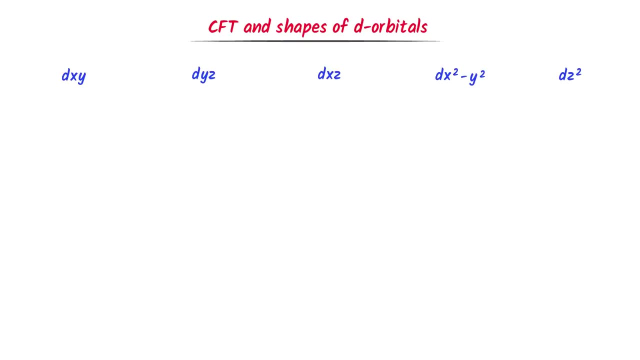 way of drawing the structures of these 5 orbitals. In case of dxy, firstly I draw x axis and then y axis. Remember that it is up to you. whatever axis you select. We know that the ship of d orbital is like double dumbbell. I draw the lobes of double dumbbell between. 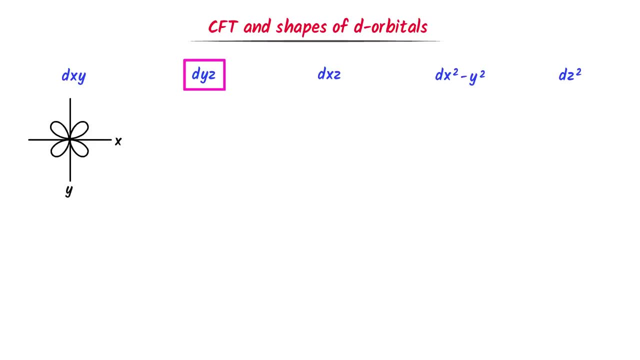 the axis. In case of dyz, I draw y axis and then z axis. I draw the lobes of double dumbbell between the axis. in case of dzx, I draw x axis and then z axis. in case of dx squared minus y squared: 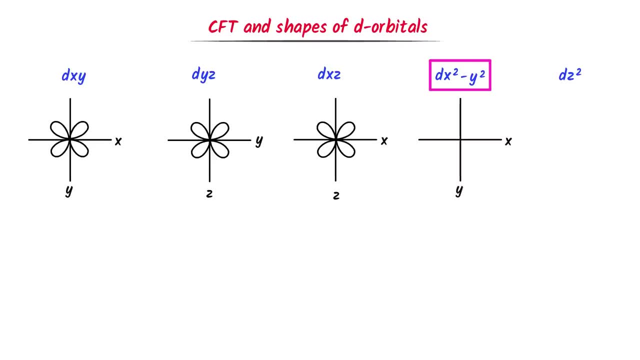 In case of dyc, the less the more In this case. also draw the dump, the 스트�ich and I draw x-axis and then y-axis Here. this squared on x and y, reminds me to draw the lobes directly on both the axes. 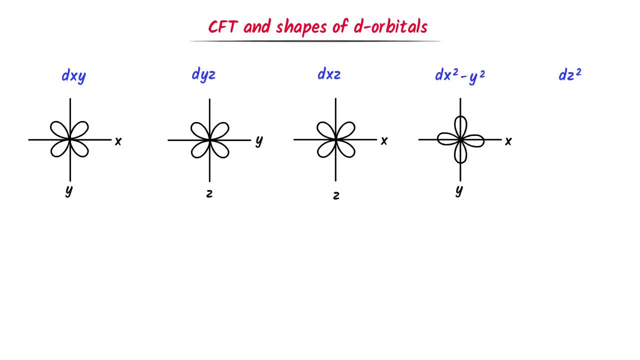 So I draw lobes of double dumbbell on the axes. In case of dz squared, I only draw z-axis. This square on z-axis reminds me to draw one lobe on axes and put a ring at the center. So these are the structures of 5D orbitals. 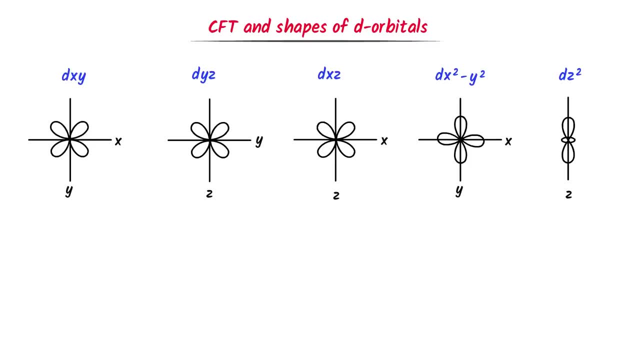 Now here are some key concepts which you must understand, otherwise you will not understand crystal field theory. Firstly, in case of these three orbitals, the lobes of orbitals are between axes, For example, like this lobe, like this lobe and like this lobe. 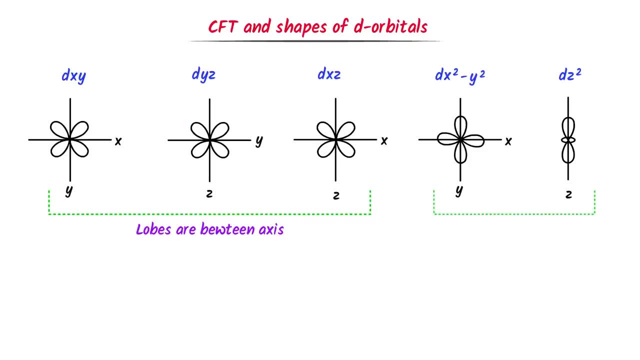 Secondly, in case of these two orbitals, the lobes of orbitals are between axes. The lobes of orbitals are along or on the axes, like this lobe or this lobe. Now, if I ask you about tetrahedral complex and octahedral complex, can you answer it? 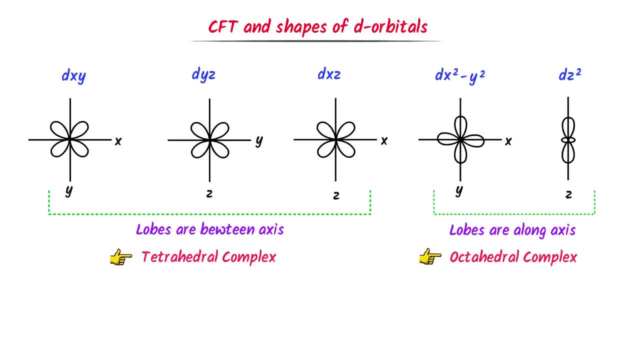 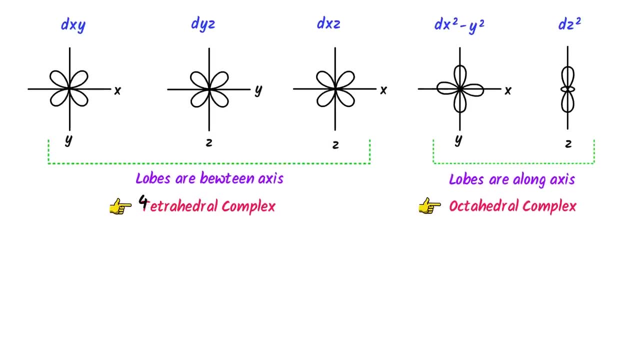 Well, the easy trick is: I select this T and tetrahedral and I write it as a 4. While I select O and this octahedral and I write it like 6.. So in tetrahedral, complex central metal atom is surrounded by 4 ligands, like COCl4-2.. 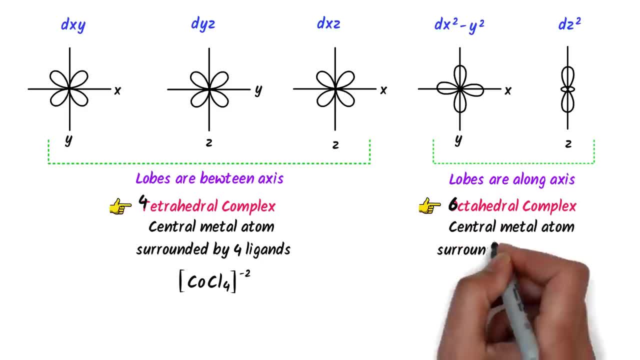 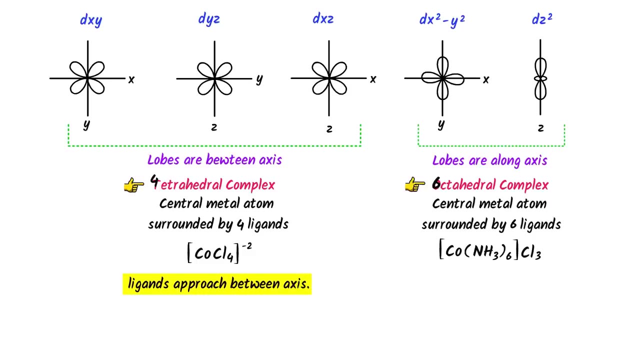 While in octahedral complex central metal atom is surrounded by 6 ligand like CONH36Cl3.. Now listen carefully: In case of tetrahedral complex, ligand approaches between axes. Let me repeat it: In case of tetrahedral complex. 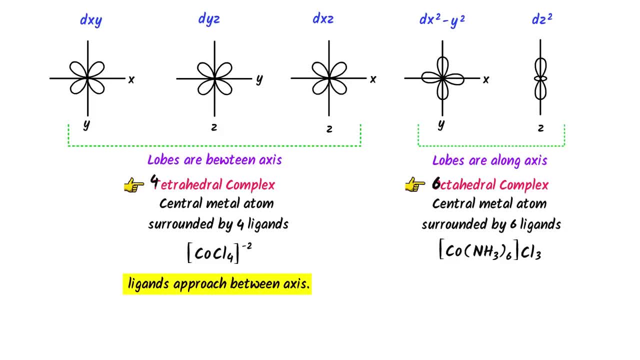 ligand approaches between axes, I mean in tetrahedral, complex ligand will attack on this lobe, or on this lobe or on this lobe of orbitals. After attack, there will be interaction between electrons of ligand and electrons of orbitals. 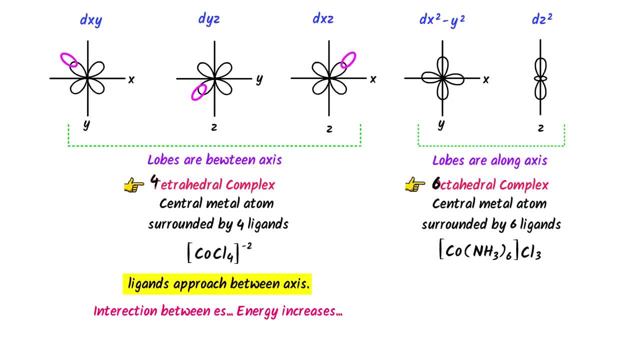 Remember that when there is interaction between electrons, energy of orbital increases. Let me repeat this important point: When there is interaction between electrons, energy of orbitals increases. When there is interaction between electrons, energy of orbitals increases. Thus we learn that energy of these 3 orbitals increases in case of tetrahedral complex. 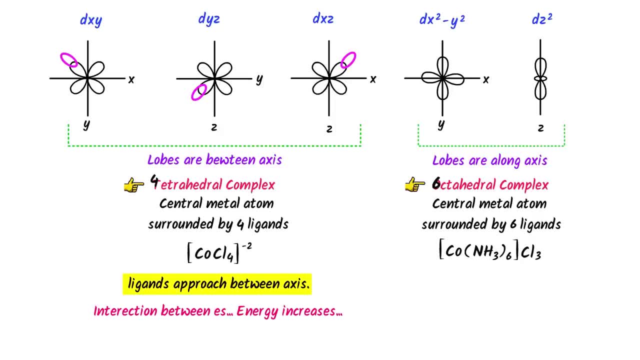 On the other hand, in case of octahedral complex ligand approaches along axes, I mean ligand will attack on this lobe or on this lobe or on this lobe- strenuous trouble I died- are on this lobe of metal orbital. After attack, electrons of ligand and metal orbitals will. 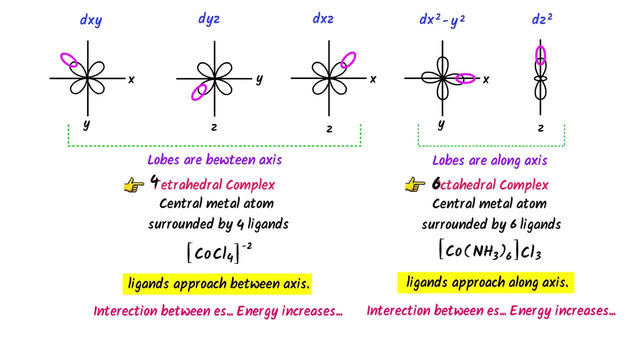 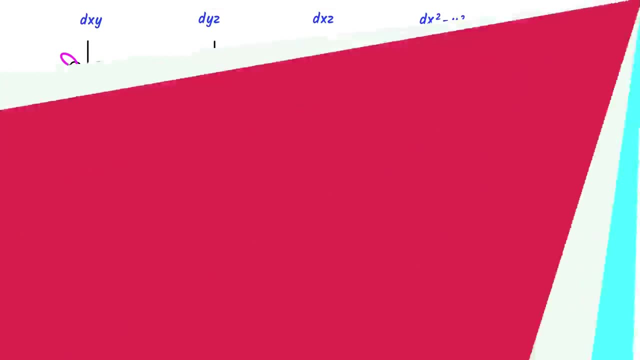 interact. hence energy of these two orbital increases. Thus we learn that energy of these two orbital increases and energy of these three orbital decreases. Thus, note down all these important points. Now let me teach you crystal field theory for octahedral complex. We already 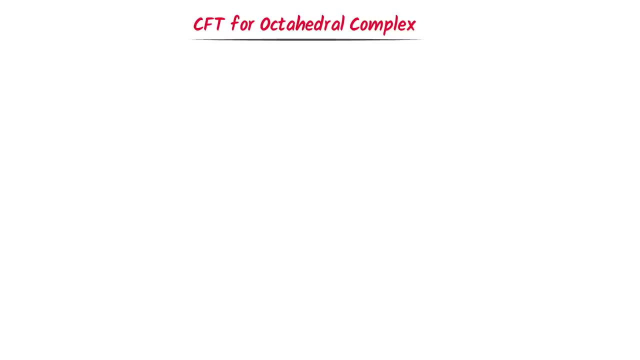 learn that in case of octahedral complex, energy of dx squared minus x squared and dz squared increases. Consider 5d: generate orbitals of a metal atom. Let a strong ligand like NH3 approach near this metal atom. The average energy of these 5d orbital increases. 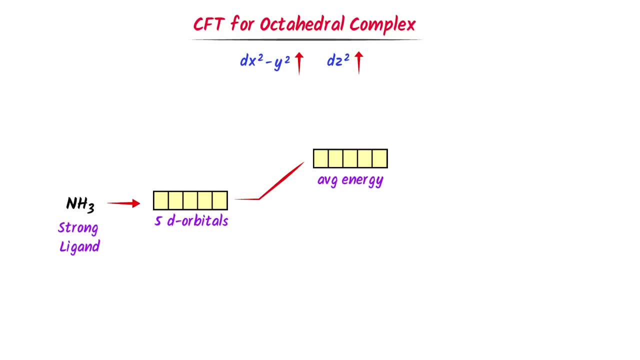 Here. a lot of students do not understand that- why energy of these 5d orbital increases. Well, I teach them a simple example. I say: when you are in danger, your adrenaline level pumps up and you get ready. Similarly, when ligand comes near to a metal atom, the 5d orbitals 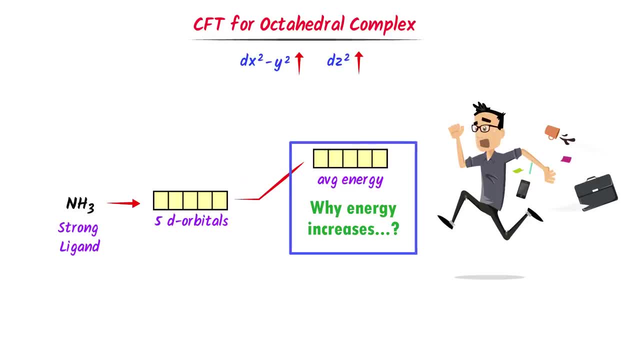 get excited and their average energy increases. Remember that in case of octahedral complex energy of dx squared minus x squared increases. Similarly, when ligand comes near to a metal atom, the 5d orbitals get excited and their average energy increases. Remember that in case of octahedral complex energy of dx squared, 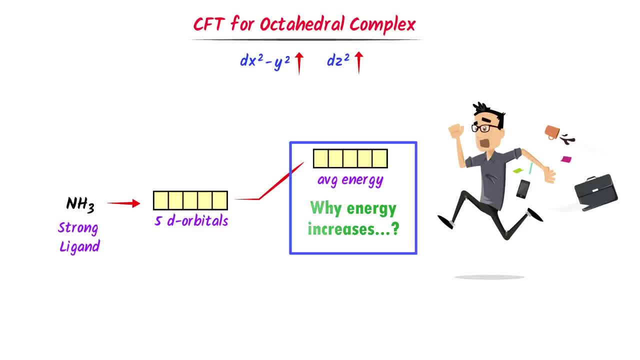 increases. Remember that I use the word average energy. Now, when ligand interacts with 5d orbitals, they split into two sets. We already learn that in case of octahedral complex energy of dx squared minus y squared and dz squared increases from average energy level because 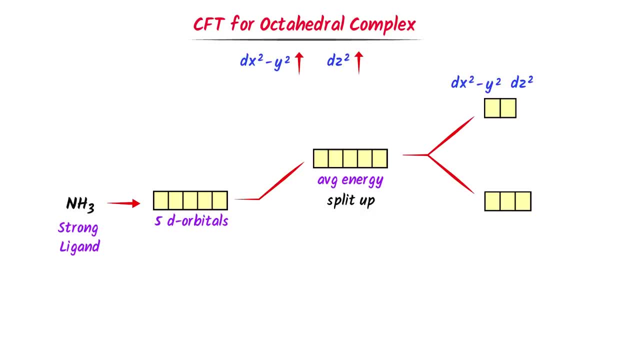 ligand like NH3, will attack along axes, While the energy of dxy will attack along axes. So the energy of dxy decreases from average energy level. We call this set of energy as eg and we call this set of energy as d2g. Remember that the energy of eg increases. 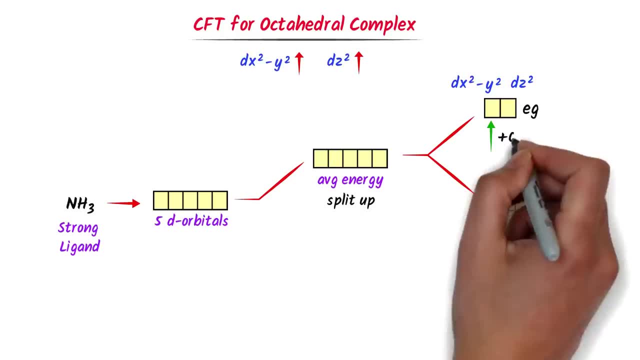 from average energy level, so its value is positive 0.6 delta. Secondly, the energy of these 3 orbital decreases from average energy level, so its value is negative 0.4 delta. We can see that this is the energy gap between these two sets of orbitals. We call this energy. 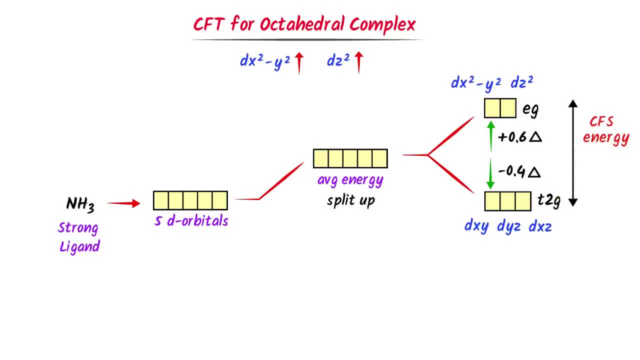 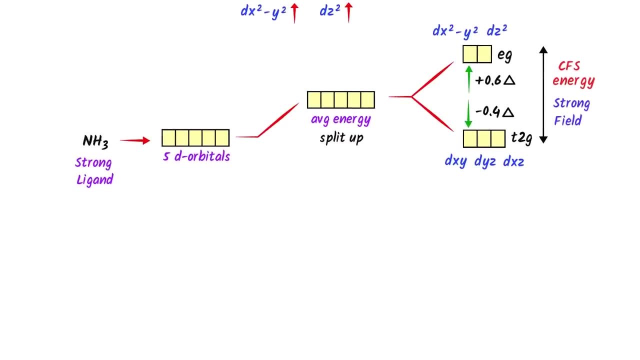 gap as crystal field splitting energy or cfs energy. Here is one important point which you must remember at any cost. Consider a strong ligand like NH3 and a weak ligand like H2O. When a strong ligand like NH3 approaches near 5d. 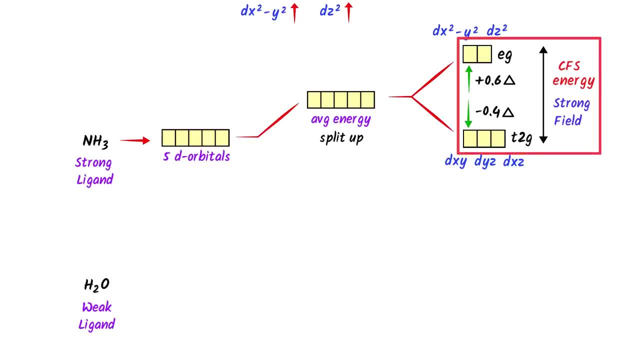 orbitals. the energy gap between these two sets of orbitals will be large. We call it as a strong field complex. On the other hand, when a weak ligand like H2O approaches 5d orbitals, the energy gap between the two sets of orbitals will be smaller and we call it. 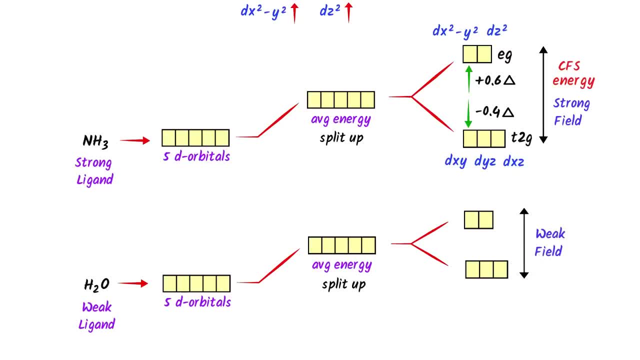 a weak field complex. Now let me teach you the electronic configuration. For example, consider that iron atom react with a strong ligand like NH3.. We know that iron has six electrons. Firstly, I fill the orbital by one electron: 1,, 2, 3.. Now the energy gap is: 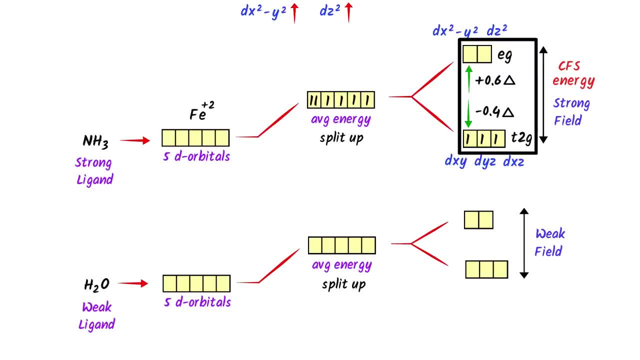 very high between these two sets. So the fourth electron will stay in this orbit, the fifth electron will stay in this orbit and the sixth electron will stay in this orbit. Now to run the electronic configuration. we know that in T2g there are six electrons, So this is: 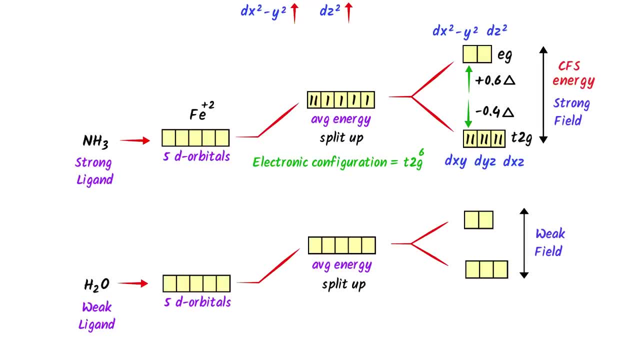 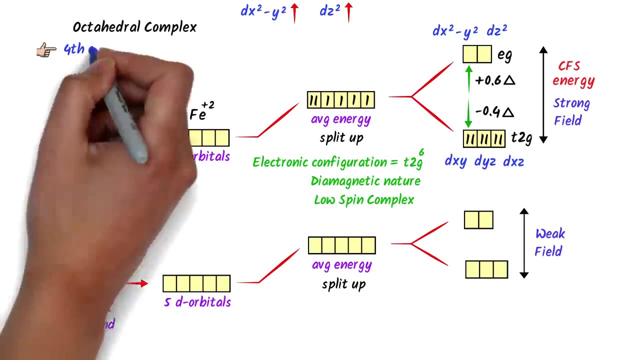 the electronic configuration for this system. Secondly, we can see that in this system the electrons are paired, So it is diamagnetic in nature. Remember that in an octahedral complex a fourth electron enters to EG. It is a high spin complex. 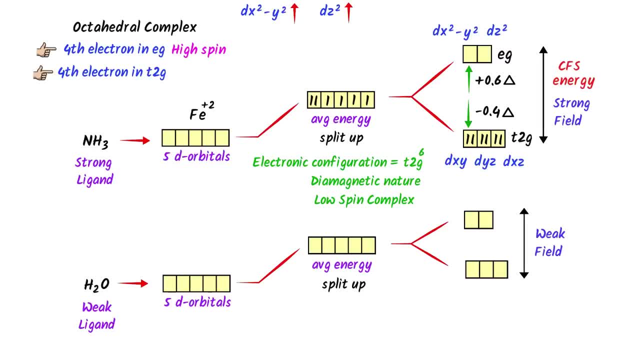 A fourth electron enters to 2g. It is a low spin complex. Here fourth electrons enter to 2g, So it is a low spin complex. On the other hand, consider that iron react with a weak ligand like H2O. We know that there are six electrons in its d orbital. Firstly, 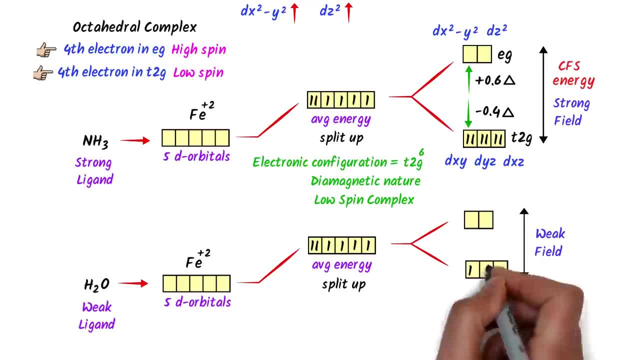 I fill the orbitals by one electron: 1,, 2, 3.. The energy gap between these two sets is very small, So the fourth electron will stay in this orbital. The fifth electron will stay in this orbital. Now all the orbitals are. 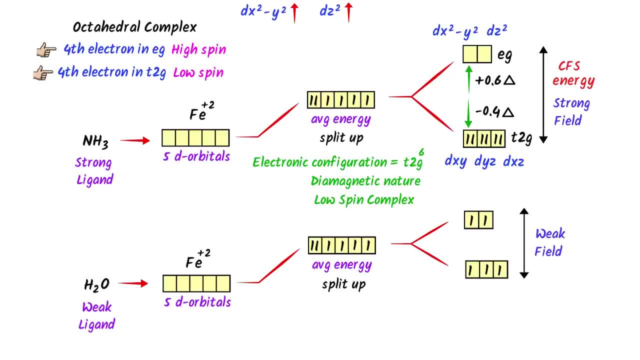 filled, I will start refilling the orbitals. I place the sixth electron in this orbital. Lastly, I write the electronic configuration for this system. We can see that there are four electrons in T2g and two electrons in EG. I write T2g4 and EG2.. So this is the electronic configuration of this system. Secondly, we 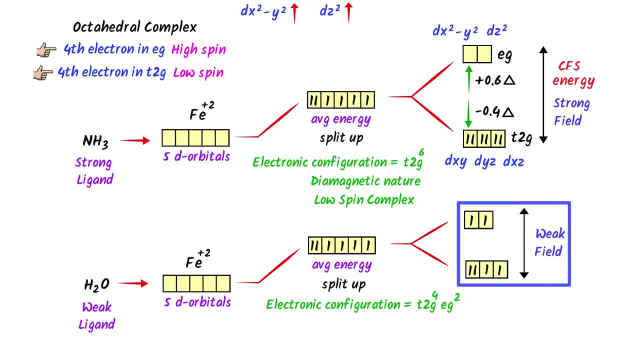 can see that there are unpaired electrons present in this system, So it is paramagnetic in nature. Here the fourth electron enters to EG, So it is a high spin complex. Therefore, using this trick, we can easily draw CFT for octahedral. 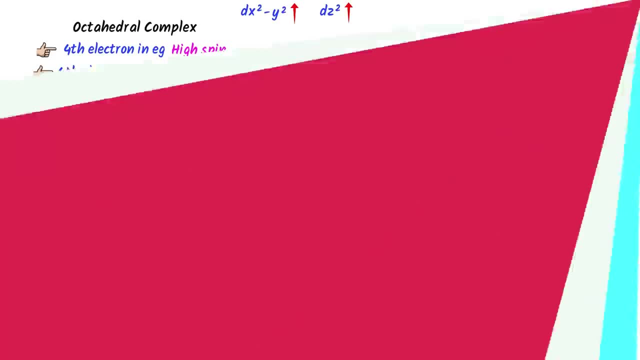 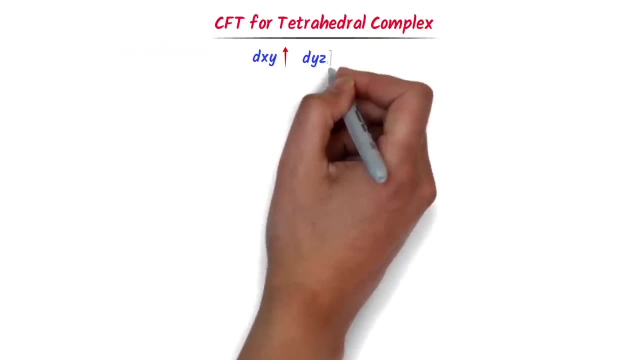 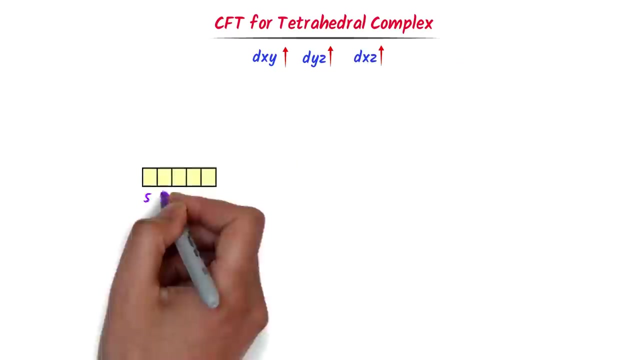 Finally, let me teach you CFT for tetrahedral complex. We already know that the energy of dxy, dyz and dxz increases in case of octahedral complex. Now consider five degenerate orbitals. Let a strong ligand like NH3 approach near these. 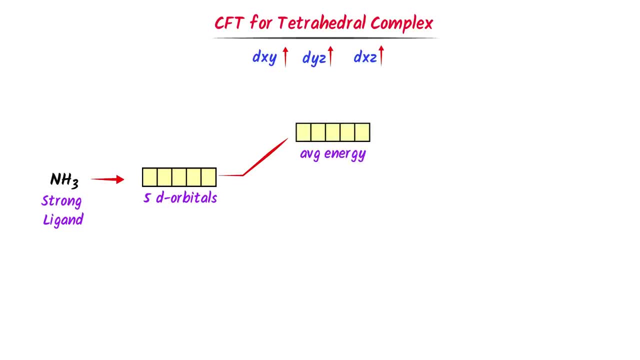 orbitals. Their average energy increases After interaction. these orbitals be put in a neutral state In the 적點化. of course these orbitals split into two sets. The energy of dxy, dyz and dxz increases, while that of dx. 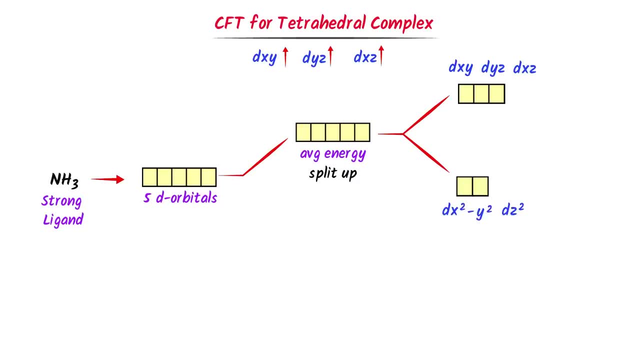 squared minus y squared and dz squared, decreases. This set is t2g and this set is eg. The energy of t2g increased, so its value is positive: 0.4 delta, and the energy of eg decreases, so its value is negative: 0.6 delta. We can see that this is the energy gap between these two sets. We call it as: 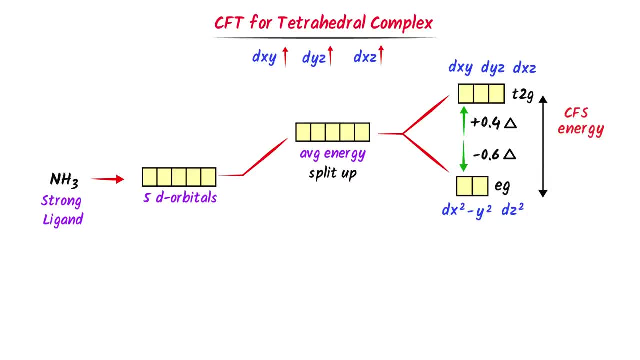 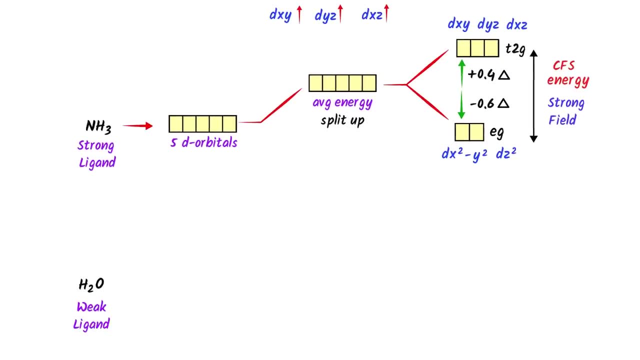 crystal field, splitting energy. Also, it is a strong field ligand. Now consider a weak ligand like h2o. We know that in case of a weak ligand, the energy gap between the two sets of orbitals will be smaller. We call it weak field ligand.